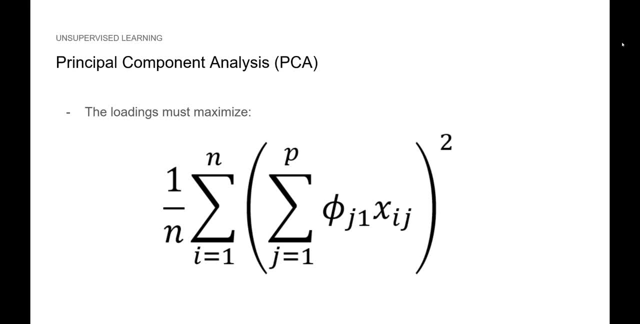 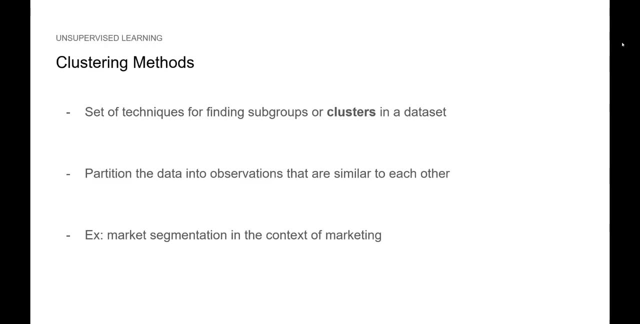 the equation you see on the screen And the sum of squared phi must be equal to one. That's it for PCA. Let's take a look at clustering methods. Clustering is a set of techniques for finding subgroups or clusters in a dataset. This helps. 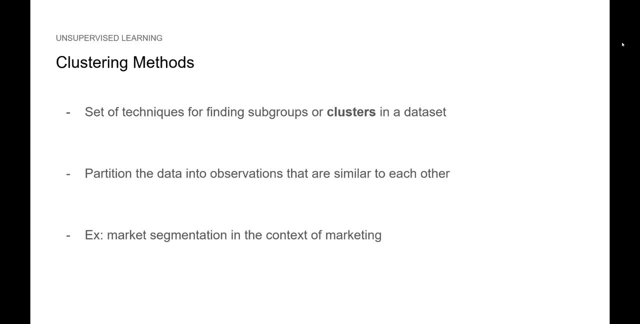 us to partition the data into observations that are similar to one another, and an application of that could be market success. Let's now take a look at market segmentation in the context of marketing. We will first explore k-means clustering, which partitions the data in a specified number of. 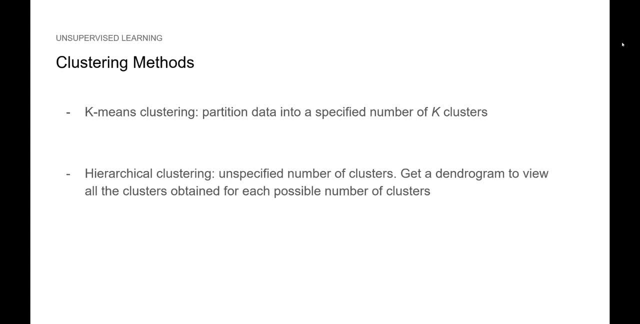 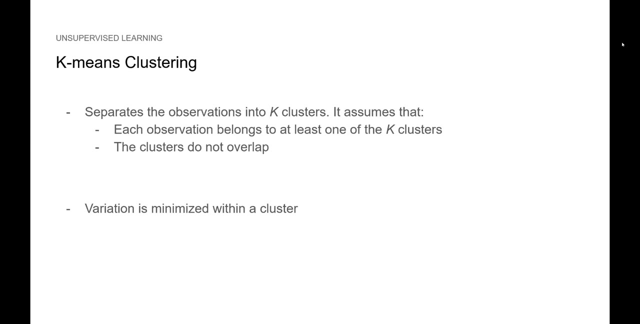 k clusters, And we will also look at hierarchical clustering, which does not need a specific number of clusters. Instead, we can generate a dendrogram and see the clusters for all possible number of clusters. So first let's focus on k-means. This method simply separates the observations. 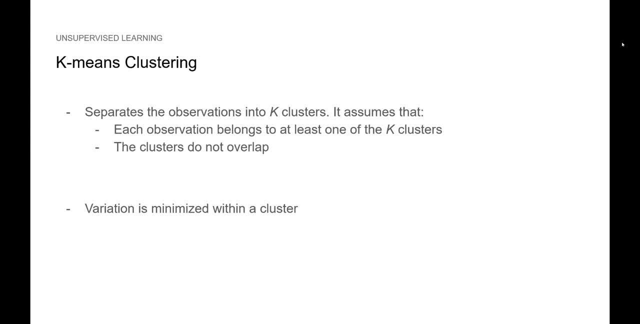 into k clusters, and we must provide that number, k. It assumes that each observation belongs to at least one of the k clusters and that the clusters do not overlap. It is important to note that the variation within each cluster is minimized. Here you can see an example of how the number of clusters will affect. 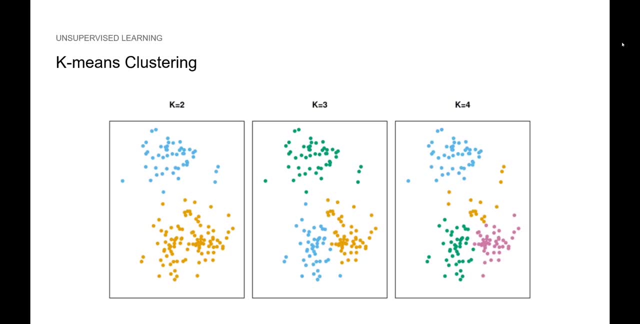 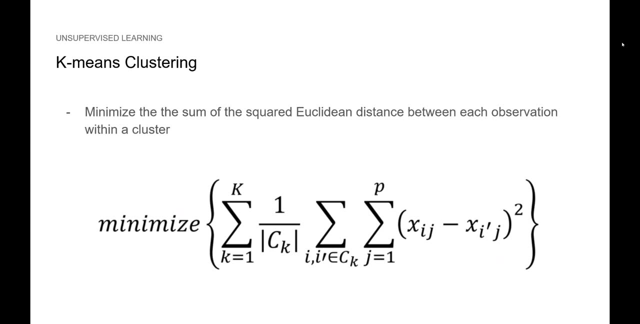 how the data is partitioned. Feel free to pause the video if you want to study this a bit longer. Clustering is achieved by minimizing the sum of the square Euclidean distance between each observations in a cluster, as expressed by the equation below. To do so, the 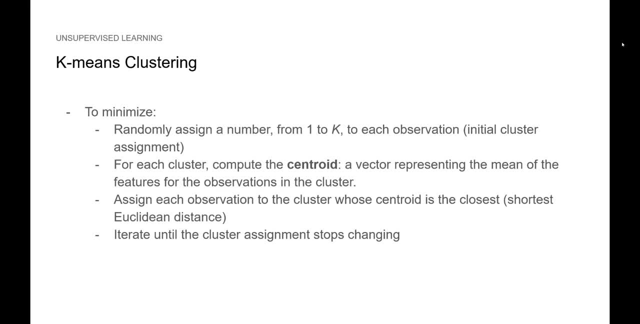 algorithm first starts by randomly assigning each observation to a cluster. Then for each cluster a centroid is computed, which is a vector representing the mean of the features in the cluster. Then each observation is assigned to the cluster whose centroid is the closest The 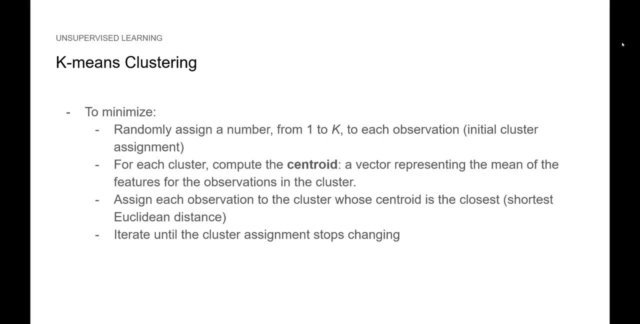 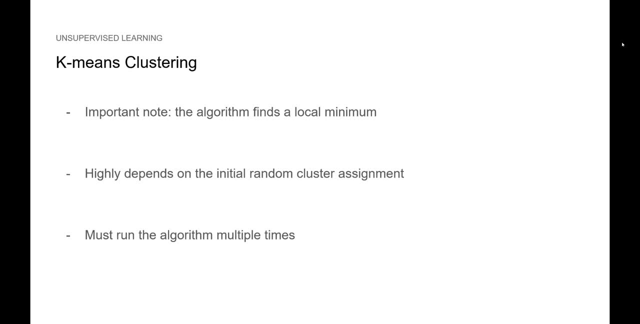 two steps above are repeated until the cluster assignment stops changing. Note that k-means will find a local minimum. Therefore, it highly depends on the initial cluster assignment, So make sure to run the algorithm multiple times to see if you always get the same results. 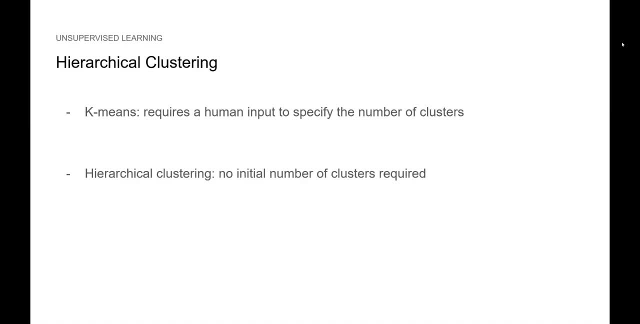 Now let's learn more about hierarchical clustering. As I mentioned, the potential disadvantage of k-means is that you must specify the number of clusters, and sometimes you simply don't know how many clusters you need. This is when hierarchical clustering comes in, because 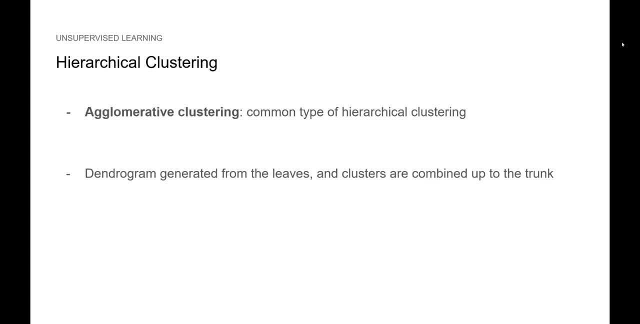 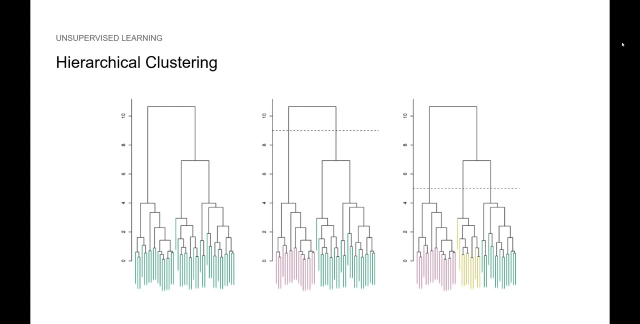 you do not need to specify the number of clusters. The most common type of hierarchical clustering is called agglomerative clustering. It generates a dendrogram from the leaves and the clusters are combined into larger clusters up to the trunk. Here are examples of dendrograms. We see the individual observations at the bottom. 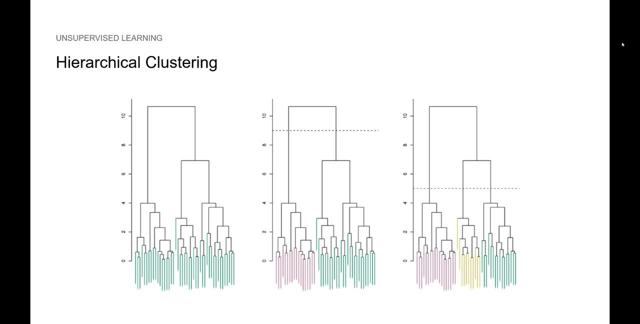 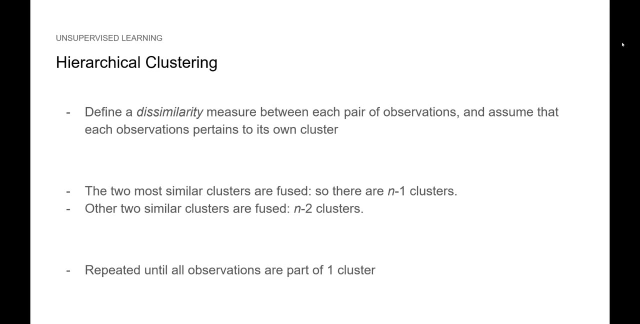 and they are combined into larger clusters as you move up in the y-axis. The algorithm is fairly easy to understand. It starts by defining a dissimilarity measure between each pair of observations, and it assumes that each observation pertains to its own cluster. 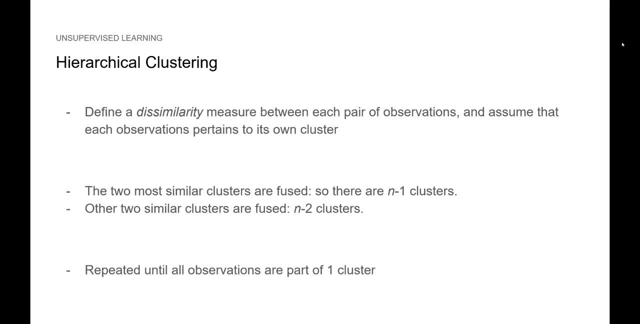 Then the two most similar clusters are combined, so they are n-1 clusters. They are combined, resulting in n-2 clusters, and so on and so forth, until all observations fall in one large cluster. Although simple, how do we define the dissimilarity measure? 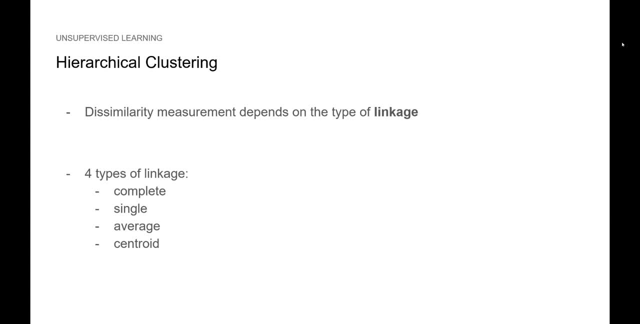 That depends on the type of linkage and there are four types: complete, single, average and centroid. Complete is also called maximal intercluster dissimilarity. It computes all pairwise dissimilarities in cluster A and B and records the largest one. With single, it's the. 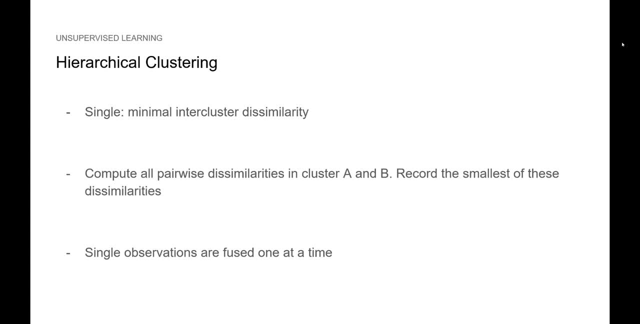 opposite, and we talk about the minimal intercluster dissimilarity. Here the smallest of the dissimilarities is recorded, and that can mean that single observations are fused, one at a time. Then we have average. As the name suggests, the average of the pairwise dissimilarities is: 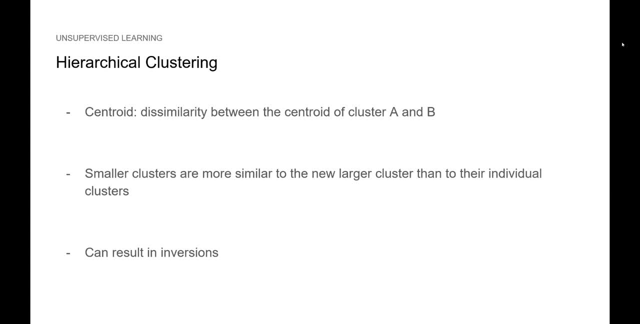 recorded. And finally, there is centroid, which computes the dissimilarity between the centroids of cluster A and B. This is sometimes a problem, as smaller clusters can be more similar to a larger one than to their individual clusters, which can lead to inversions. Complete average and centroid. 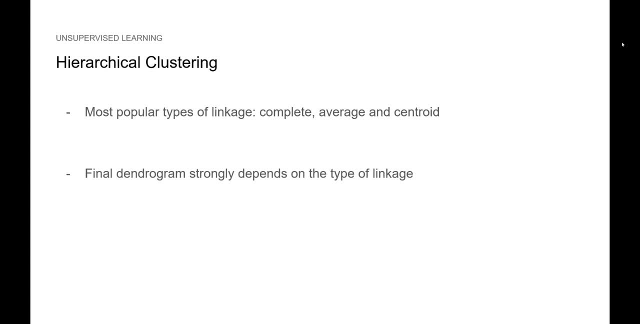 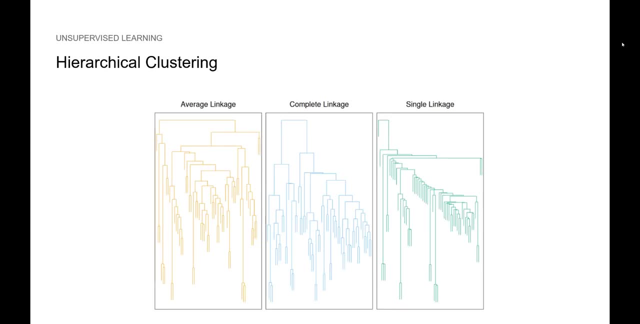 are definitely the most popular types of linkage. Note that the final dendrogram highly depends on the linkage. As you can see here, average and complete are pretty similar, but with single linkage the dendrogram is quite unbalanced and that's why this method is not used often. 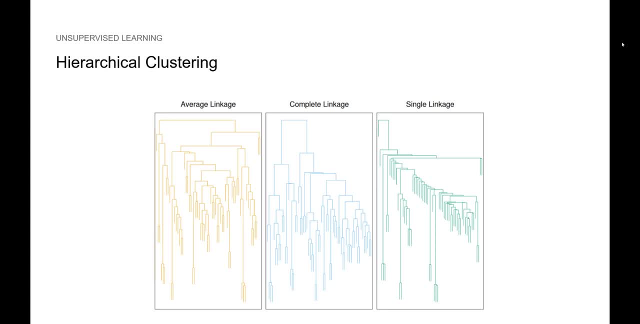 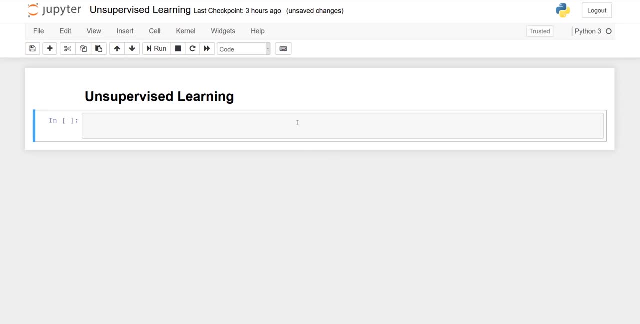 You can also see the individual observations being merged into larger clusters. That's it for the theory. Let's get coding now. Let's apply what we learned in Python now. These exercises are available as examples on the sklearn website. I am simply reworking them a bit or explaining them here. The links are in the. 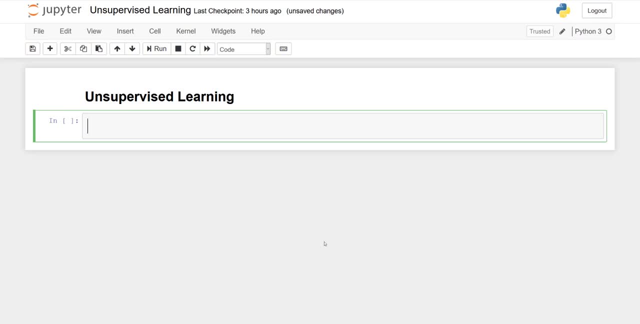 description, and the complete notebook on GitHub is also in the description down below. We'll start off by importing some libraries. We will need numpy, We'll also need matplotlibpyplot as plt And finally, from sklearnutils we will import shuffle. 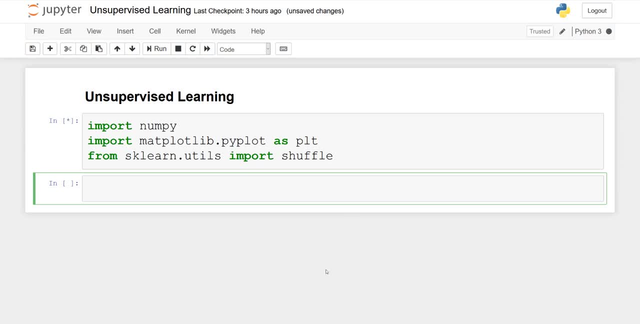 So let's kick off this tutorial with a clustering. We will do color quantization with k-means, which is a technique to reduce the number of colors of an image while keeping the integrity of the image. So to do that- we will learn we will need from sklearndatasets import load underscore sample. 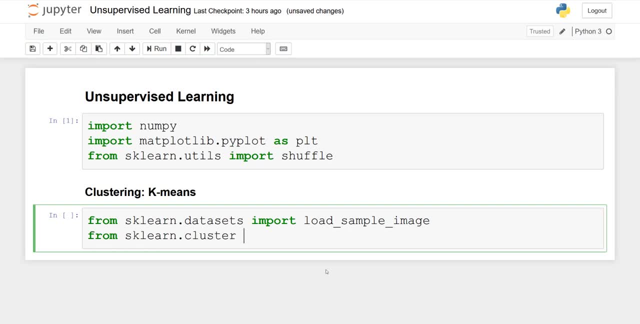 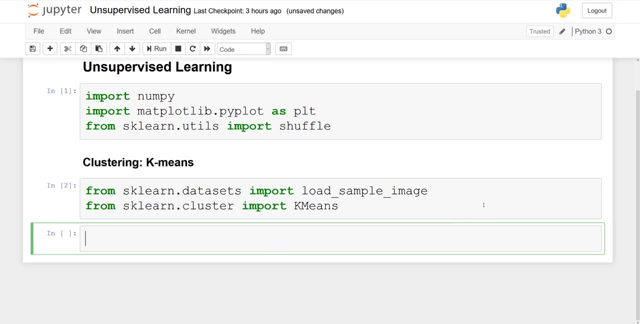 underscore image. and from sklearnutils: import image from imageimg: import load underscore sample underscore image. and from sklearndata sets: import load underscore sample underscore image. and from from sklearncluster. We will import k-means Now, after importing our libraries, we will load. 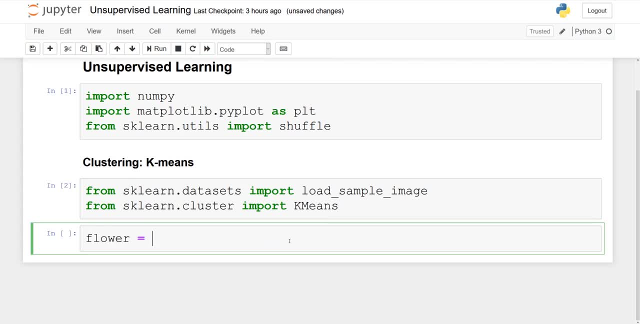 the image of a flower, So the flower will be equal to load sample image and we will pass in the name of the image. In this case it is flowerjpg. Now we need to convert to floats and divide by 255, because colors are expressed as RGB- right, Red, green and blue, with values. 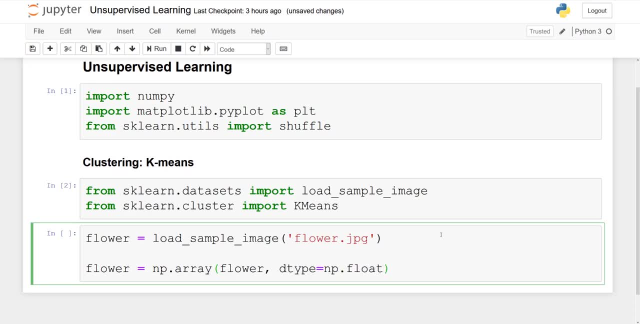 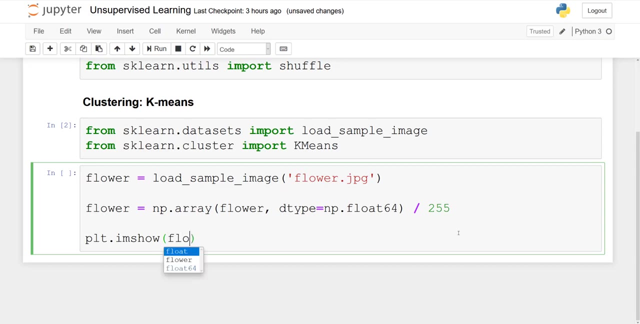 from 0 to 255.. So we need to normalize that so that the image displays correctly with matplotlib. So this is what we are doing here, So we convert to floats and we divide by 255 to normalize everything. Finally, we can show the image with pltimshow and we pass in flower. 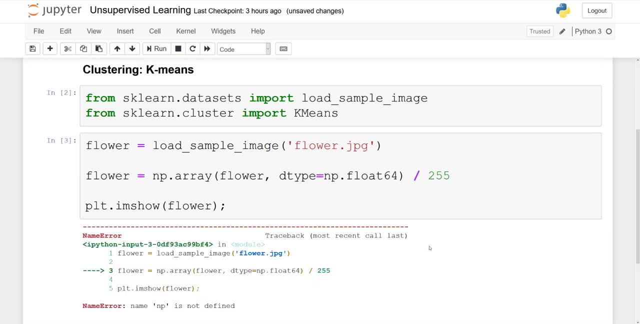 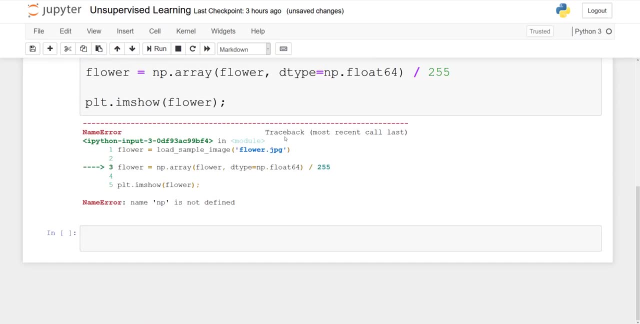 Now we will import the image of a flowerjpg. Now we need to convert to floats and divide by 255. Now I have made a mistake here. The name np is not defined. That's because I did not import numpy as np. Sorry about that. So, after rerunning this cell and rerunning this cell, here we finally get. 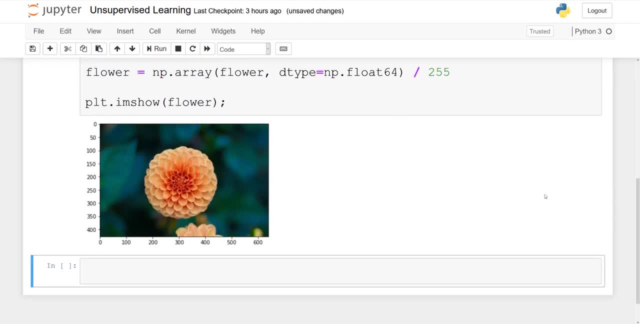 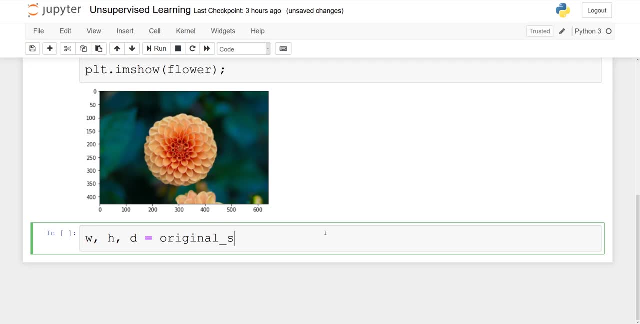 the picture of our flower And this is what you should get. Now we will change the image to a 2D matrix, So width, height and depth will be equal to original shape, which is a tuple of flowershape Here. 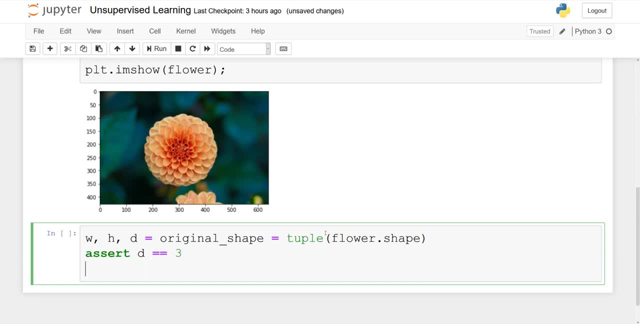 d is the depth will be 3 because, as I explained earlier, each layer will correspond to either red, green or blue, So three values in this case. And now we reshape it, So imageArray is equal to npreshape flower, and then we'll reshape with the width times the height. 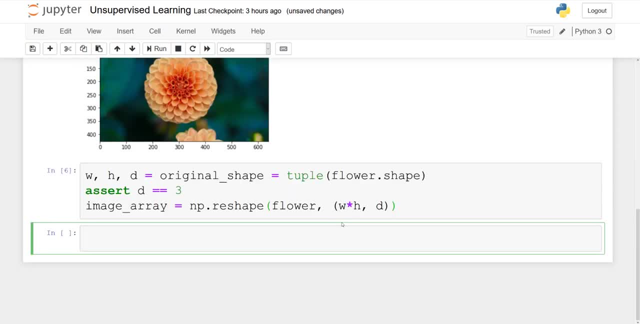 And the other dimension will be the depth. Awesome, Now we will reduce the number of colors to 64 by running the k-means algorithm, where k will be set to 64. So our image sample will be equal to shuffle the image array. 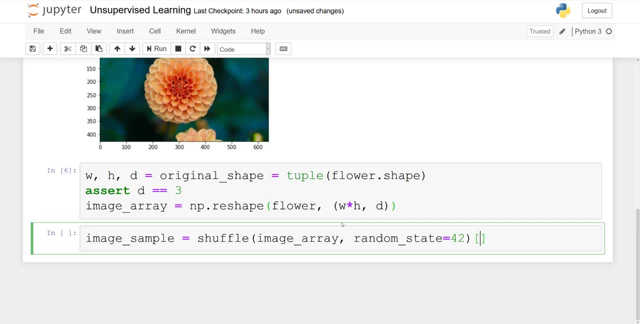 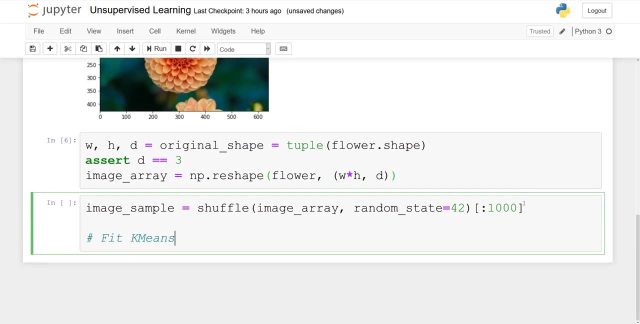 We'll give it a random state equal to 42 so that the results are constant whenever we rerun the cell, And we'll take the first 1000 samples. Now we will fit the k-means algorithm And we set here the number of colors. As I said, this will be equal to 64.. 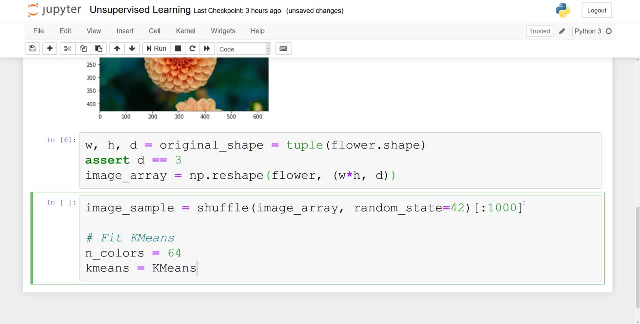 Then k-means will be equal to k-means. We initialize the model, We pass in the number of clusters, which is the same as the number of colors in this case, And again the random state equal to 42 because, as you know from the theory part, k-means starts by randomly assigning. 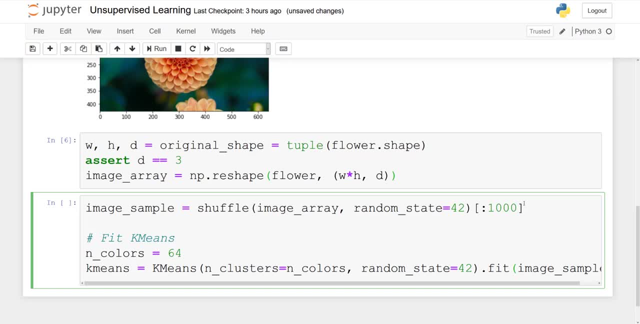 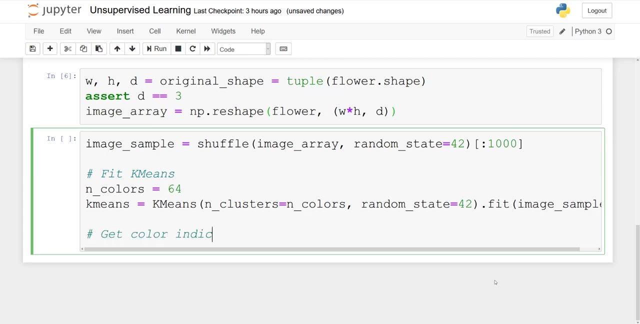 each observation to a cluster. So we keep the random state equal to 42 to give the same results every time. And then we simply fit the algorithm. And then we simply fit the algorithm. Then we get the indices for each color for the full image. That will be useful when we need to. 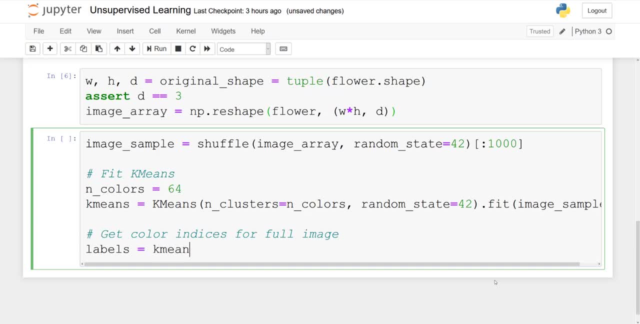 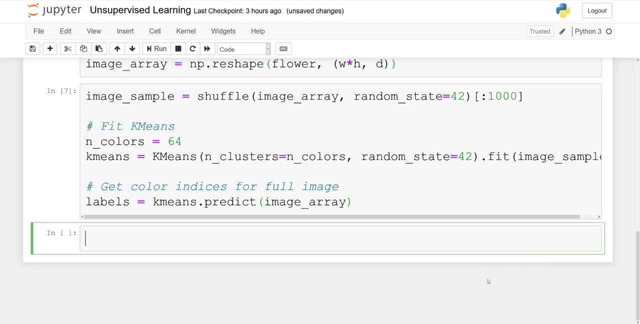 reconstruct the image right. So each pixel in the 2D array will be assigned to a certain cluster And that will help us to bring back the color and rebuild the image. So it's simply the labels, which is a prediction from the k-means. Now we need to write a function to rebuild the image. 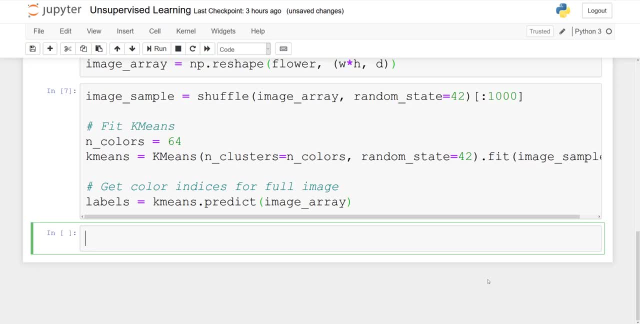 So, like I said, we're going to use the k-means algorithm to do that. So we're going to use the k-means algorithm And, like I said, each pixel is assigned to a cluster which corresponds to a specific color. 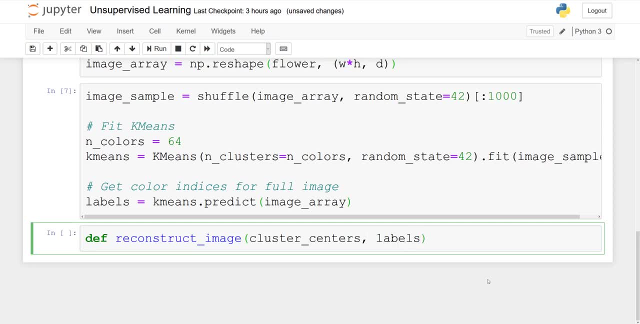 So we define, reconstruct, underscore, image And we will need as parameters the cluster centers. We'll need the labels And we pass in the width and the height of the picture. So d will be equal to the cluster centers dot shape And we take d at index one. 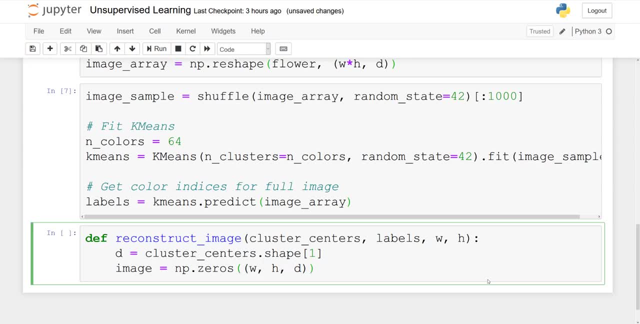 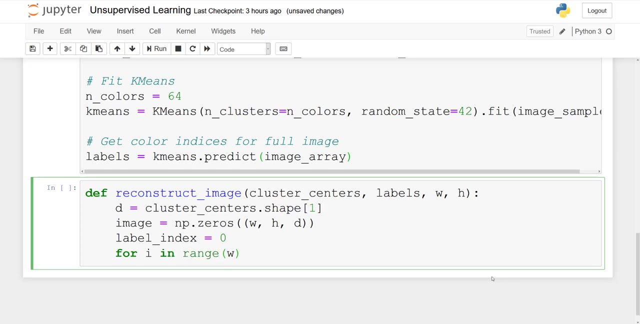 Then the image will be simply an array of zeros, in this case, And the shape will of course be the width, the height and the depth. The label index will start at zero. So that's pulled out. and then let's take w to be equal to w. 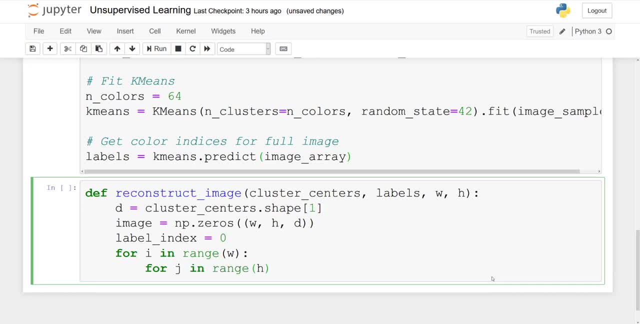 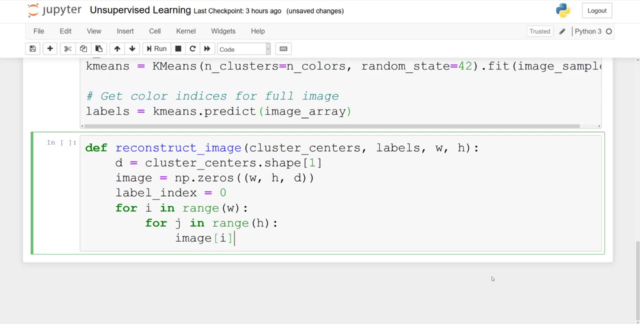 And then for i in the range of the width And for j in the range of the height. We write that image at index ij. So this is, the coordinates in the 2D matrix Will be equal to the cluster centers at labels and that itself will be at the label index. 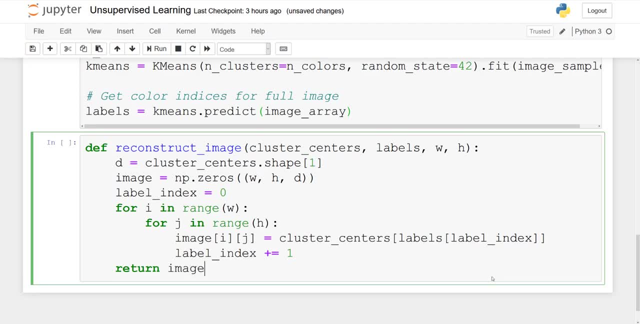 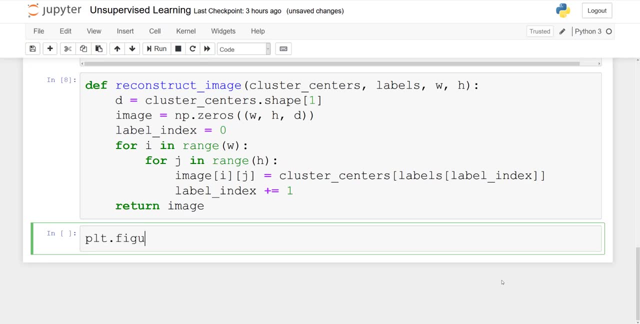 And then we increment the label index, so plus equal one, and finally we return the reconstructed image. So that's it for this function. Now we are ready to display both the original image and the reconstructed one, with only 64 colors. So the first plot will be the original image. 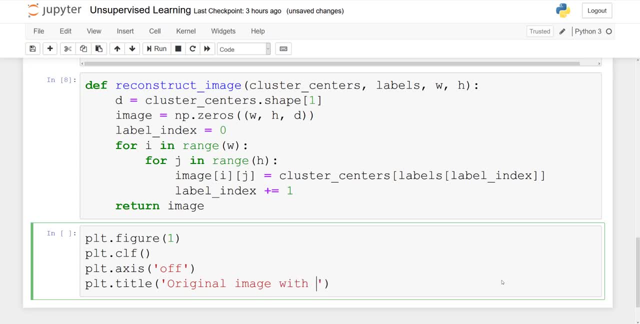 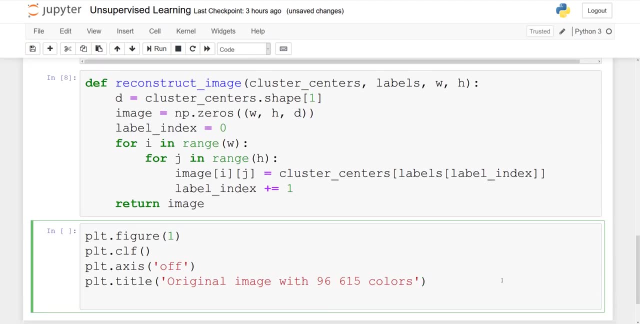 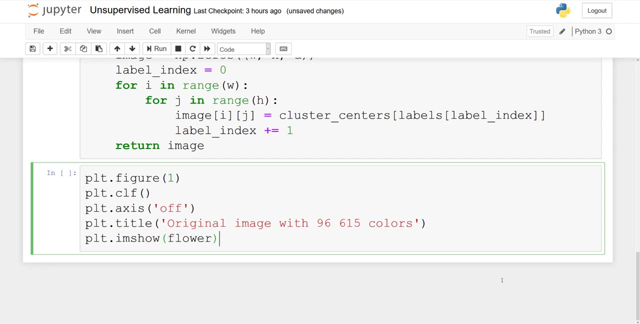 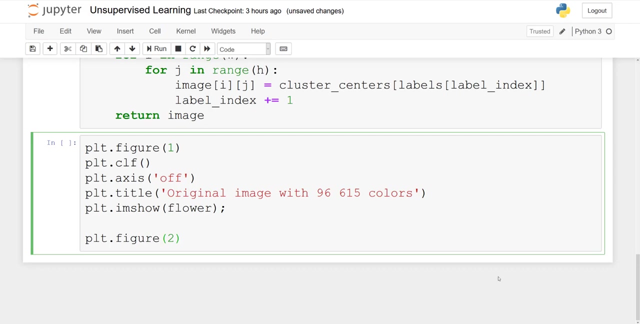 So we'll turn off the axes and then plttitle will be the original image With 96,600 pixels, 215 colors, And then we will show the original image, which in this case is simply flower. And now our second plot, so pltfigure2.. 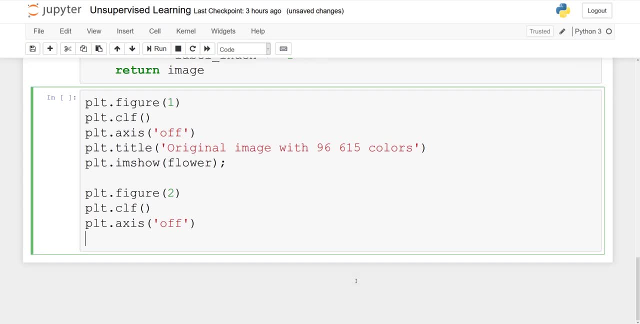 Here we will display the reconstructed image. So again, turning off the axes, The title will be Here. we will write a string, actually we'll pass in a parameter in this string. So reconstructed image with n colors, Because you can change the number of colors. we will do that after. 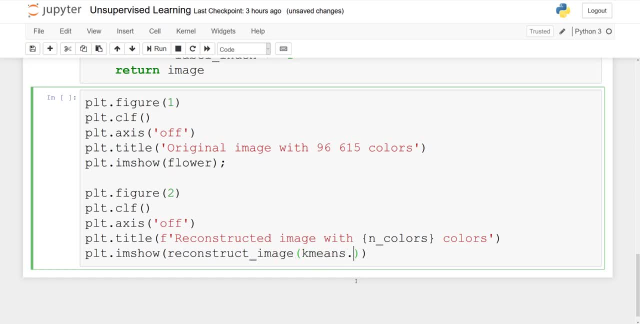 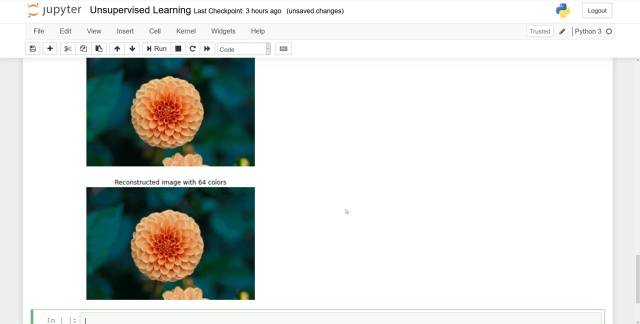 And then we show the reconstructed image. So in there we will pass in our function Reconstruct image And you pass in key Key means, dot, cluster, underscore, centers, underscore, Pass in also the labels And you pass in the width and the height that we defined earlier. 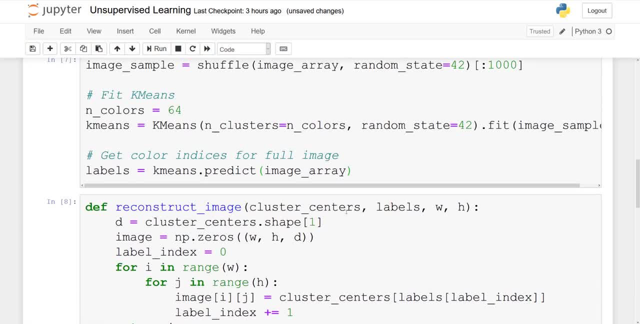 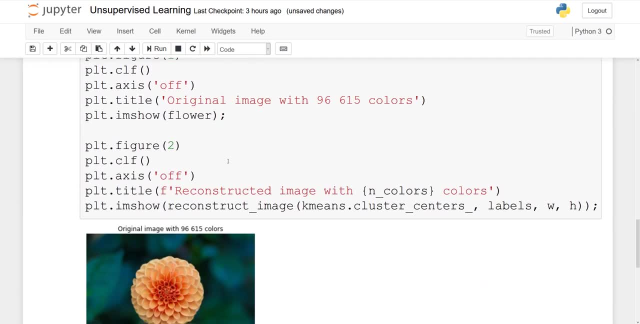 And you get the following result. So, as you can see, the integrity of the image is kept. Actually, the flower itself is very similar. I would say that only the background is very different. So let's go above and change the number of colors, just for fun. 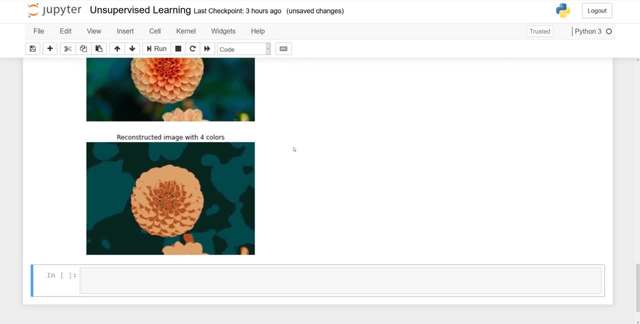 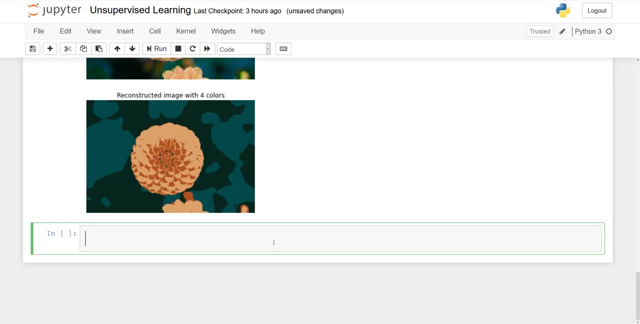 So let's say we want only four colors. So we're running these cells. As you can see, now with four colors the image is very different, But you can see it's almost like an artistic effect that you can play around with. So feel free to play around with this number of colors with yourself. 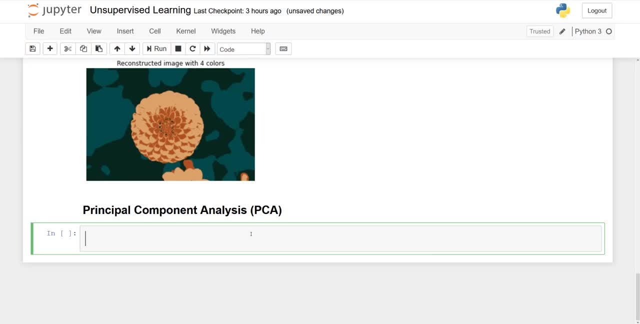 Now let's work with PCA for dimensionality reduction. Here we will work with the Iris dataset. This dataset has four features, About three of them, Three different kinds of iris flowers, And our goal is to visualize the dataset in two dimensions. So from sklearndatasets we'll import load iris. 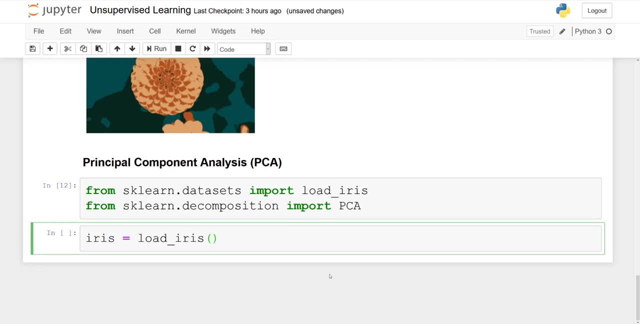 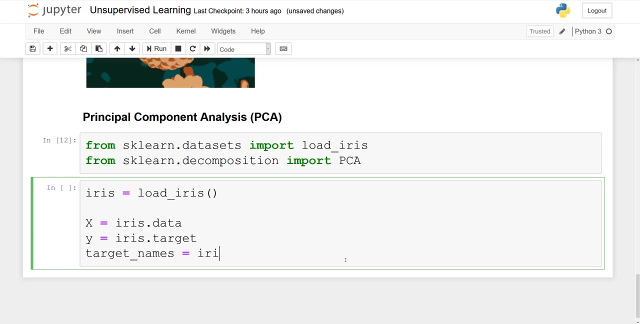 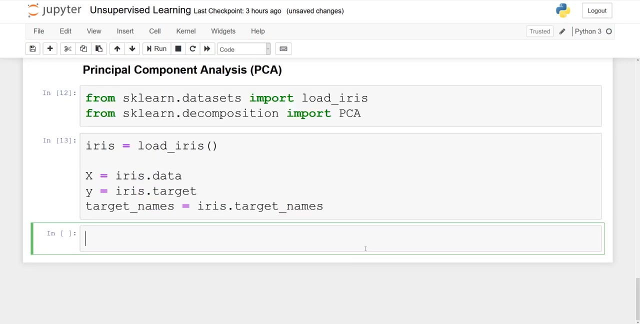 And from sklearndecomposition import PCA. Now let's load the iris dataset, So iris will be equal to load iris. The features is irisdata, The target is iristarget And then the labels or target names. here is iristarget__names. 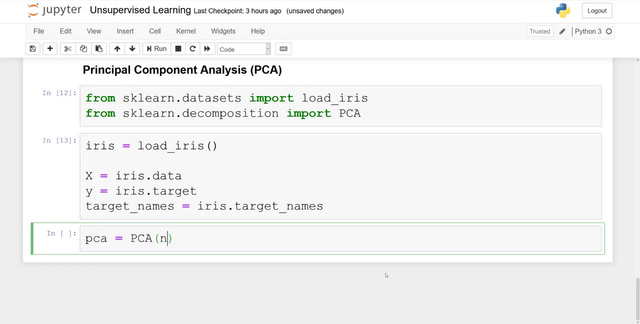 Awesome. Now let's initialize the PCA algorithm And we will specify that we want only the first two principal components, since we want a 2D plot. Then x__r is pcafit, And then x__r is pcafit, And then x__r is pcafit. 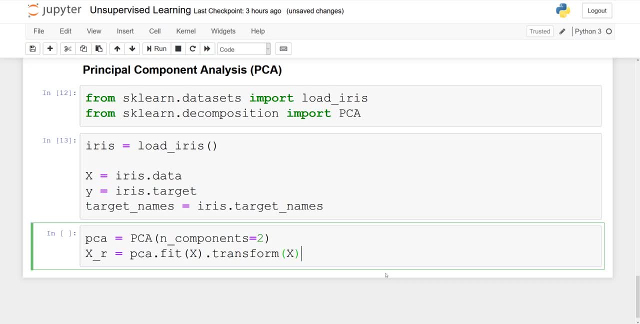 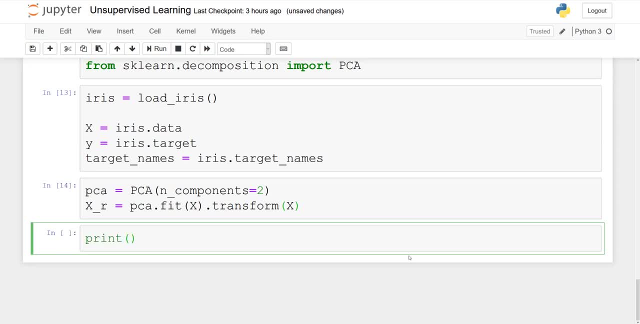 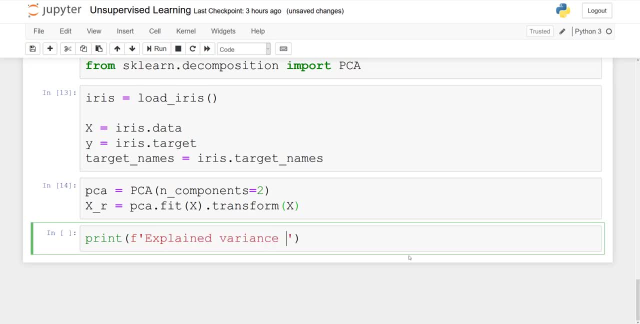 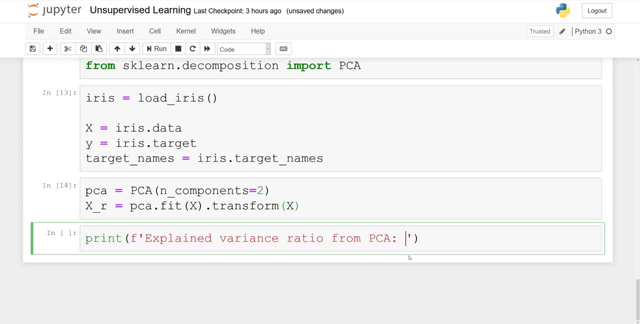 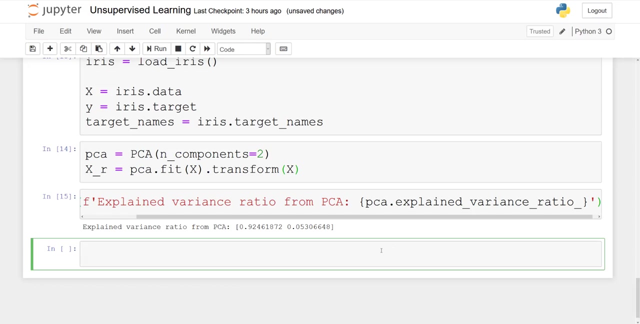 And then x__r is pcafit. So the explained variance ratio from PCA and you can extract this information from the PCA object itself. so it's PCA dot EXPLAINED. underscore VARIANCE underscore RATIO. underscore Running this cell. as you can see, the first principle component explains 92% of the variance. 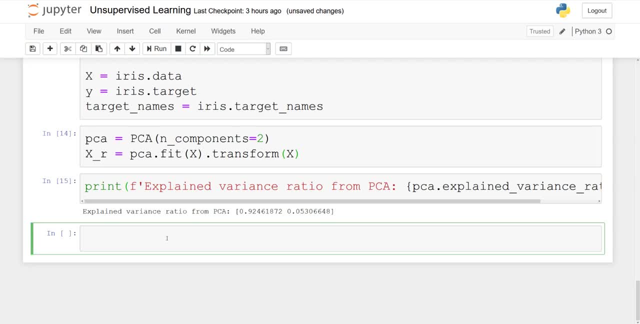 the second one 5%. So that means that a total of 97% of the variance is explained with only two components. So now we are ready to plot our data set in 2D and that newly transformed data contains about 97% of the variance of the original data set. So here we'll just specify: 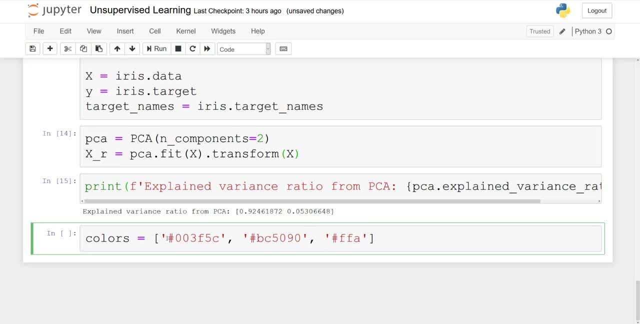 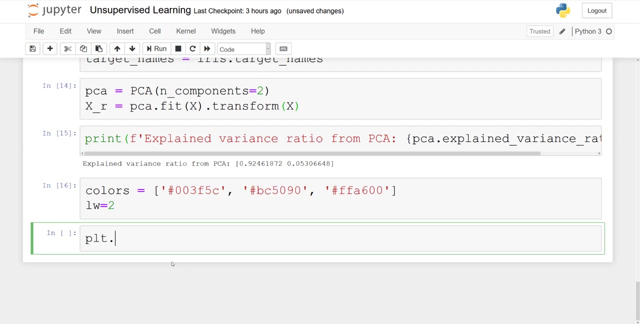 three different colors to distinguish between the three different kind of iris flowers. So the final one will be FFA600 and we'll set the line width equal to 2.. Then pltfigure and then for color in: oh sorry, so for color i target name in zip. 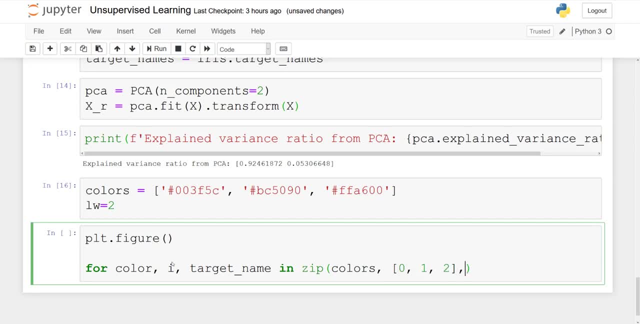 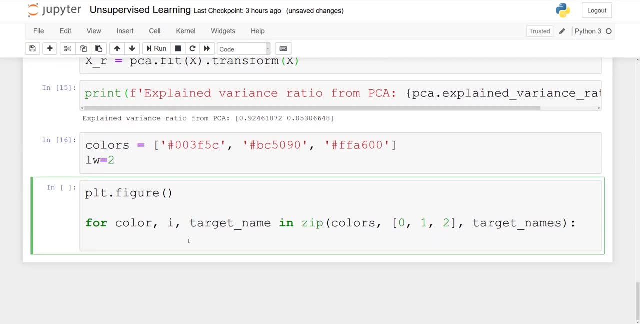 and we pass in colors. we will pass in 0, 1 and 2 and we pass in the target names. so 0, 1 and 2. here are simply the, the classes, right? so we'll draw a scatter plot. so pltscatter xr when y is equal to i.